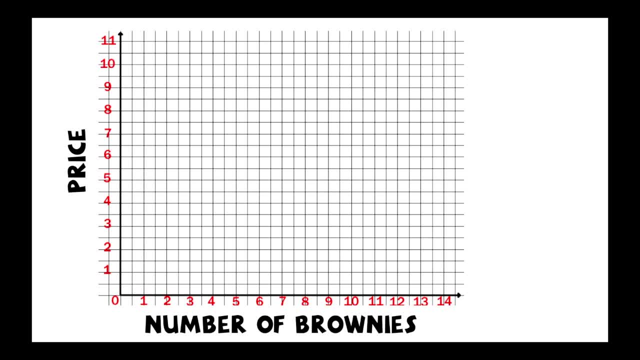 First, I need a graph. So if we were to graph this relationship, you can see a couple of things. If we had one brownie it would be 50 cents. So on this graph, number of brownies is one and I go up and when I go over, 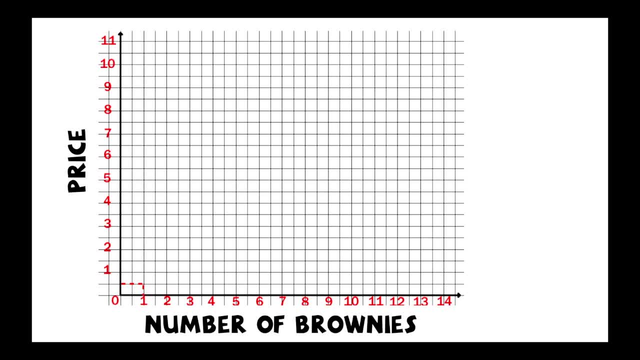 to the left, I'll see that it actually says the price is 50 cents. We know also that if we were to buy 10 brownies, it's five dollars. We found that calculation in the prior video on rates. It makes sense. It's half the price. Well, if that's the case, if I have six brownies, it would be three dollars. 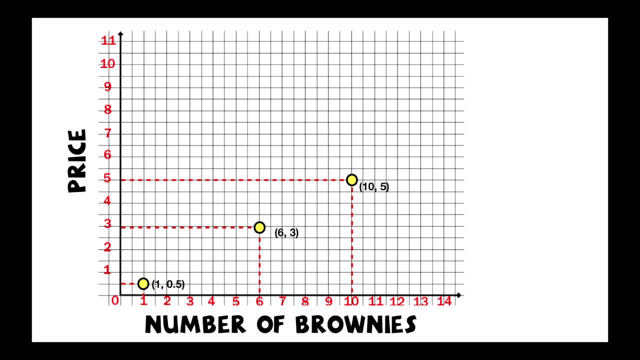 So look at these points. I have one point, five, six, three and ten five. They all show the ratio relationship between the number of brownies and the price. The number of brownies here is the independent variable, because the price will depend on how many brownies I actually buy. but the cool thing about this is that if I 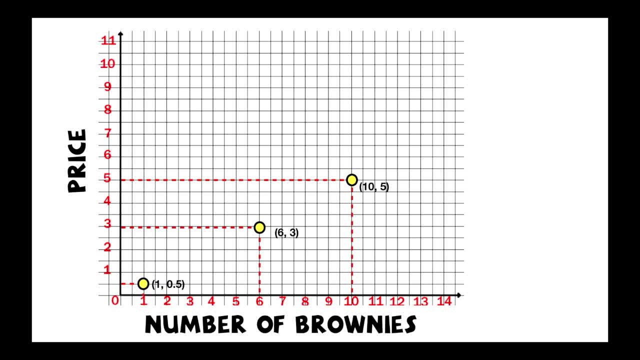 actually connect all the brownies together- which is why I have a lot of brownies- and if I actually connect all these points together is forming this nice line that will help me determine other relationships between the number of brownies and the price, For example. let's say I wanted to. 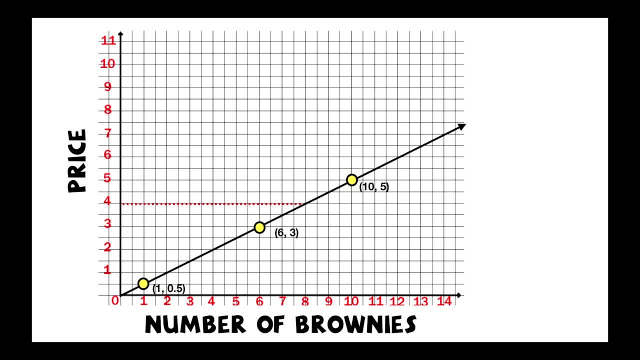 figure out how much I can get for $4.. How many brownies can I get for $4?? Well, using my graph, I could go across and see: oh well, hits the $4 at the line right about there If I go straight. 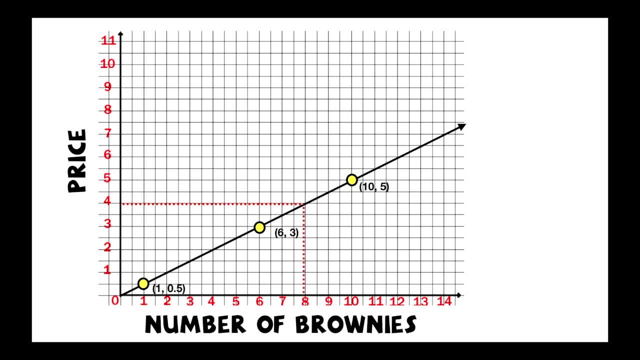 down, I could get eight brownies for the $4.. Maybe I want to figure out how much money it would be if I bought five brownies. So if I bought five brownies, according to this graph it would cost me $2.50.. So the graph really helps me figure out mathematical problems. 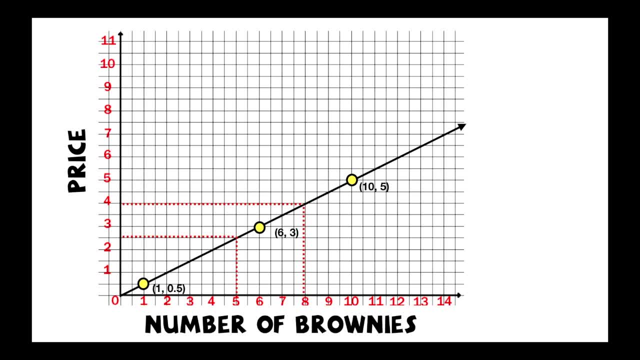 just using the ratio relationship, the proportional relationship between these values. So this graph is actually directly proportional, meaning that the values are very proportional to each other, And I know this because they actually go through the origin zero, zero. So each value. 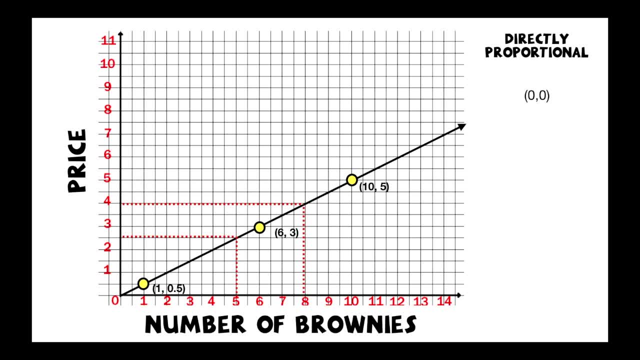 in this line has the same type of relationship. It's in proportion to each other. This must also have some sort of linear relationship, And I know this because there's a line. And that's what linear means. It means that they lie on the same line. 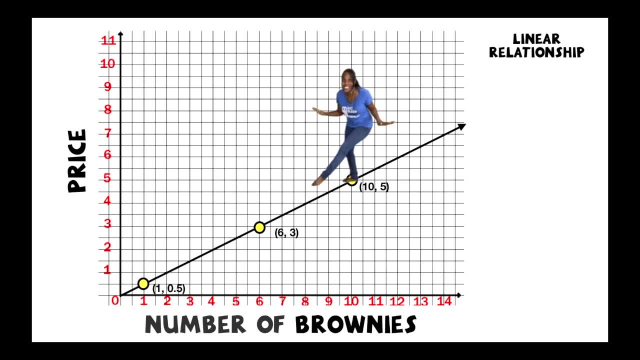 the same straight line And these points lie on the same straight line. If there is a linear relationship, that means there must be a pattern, a pattern of values that I can follow to look at this relationship. So, if you notice, there is a pattern Going from each dot, each level of this, 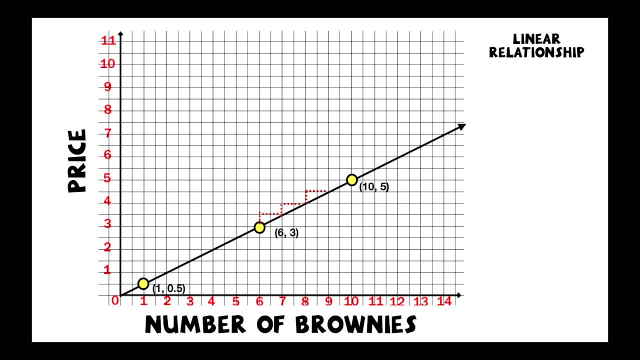 line I go up one and over to the right two, up one and over to the right two. If I follow this pattern, I will actually hit every point on this line. This pattern is the slope of this line. It's the rise over the run. 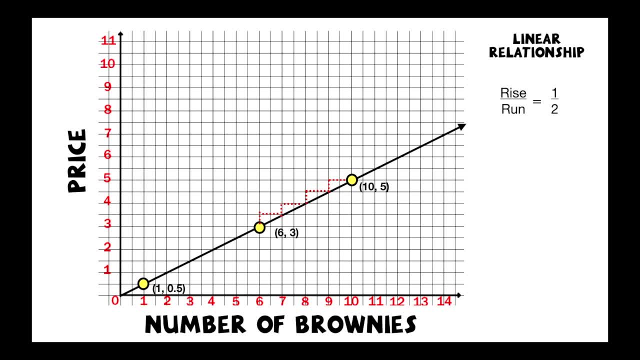 In our case, the rise over the run is one over two. Every linear relationship has a slope, has a value like this. It might not be the exact same numbers, but it has a rise over run type of value. This value is also great to show how the price is: half of the amount of brownies. 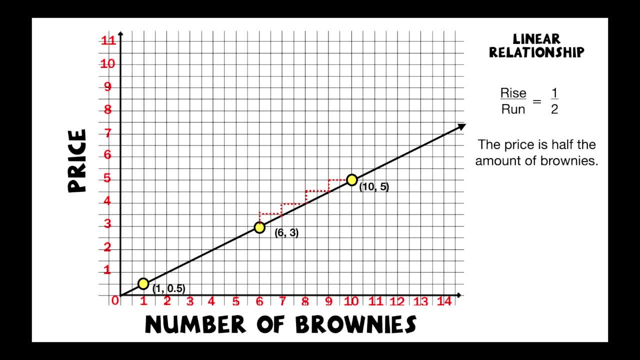 Think about it: If I had six brownies, the price was three. If I had 10 brownies, the price was five. The slope is showing that relationship, that it's half the price of brownies And once again it's going through the origin of. 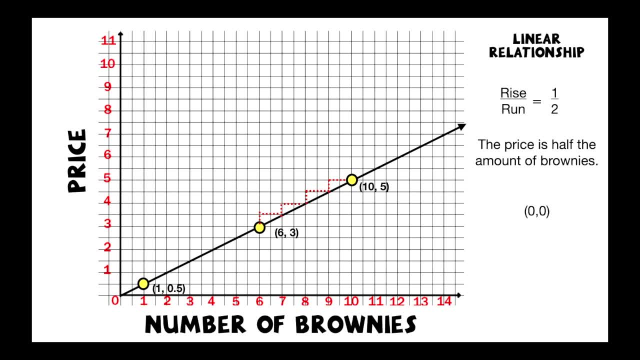 zero, zero. So I could use this to form an equation that would signify the line, the actual linear relationship. So my X is my independent variable, That's the number of brownies, And my price is Y. Okay, So if my price is half of the number of brownies that is shown by the equation, Y equals. 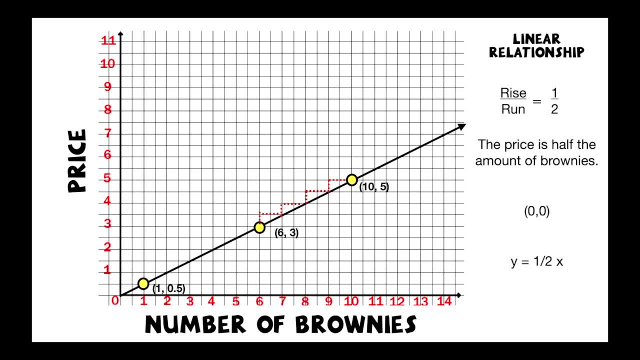 one half X, because I had to take the number of brownies which is my X multiplied by a half to get the new price of Y linear relationships. It's really cool, But what if something happened? What if, instead of just the price being half the amount of brownies, what if I got a deal? 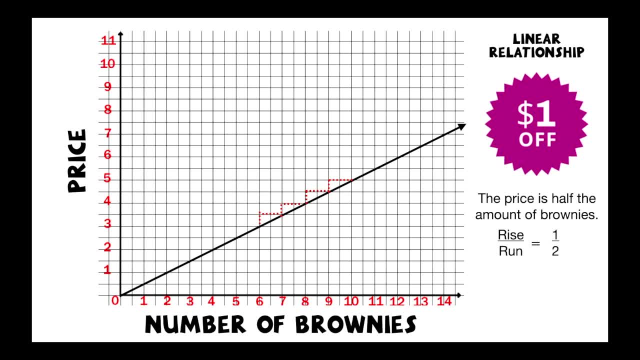 What if I have a deal where the amount of brownies actually had a? I had a coupon and I found the amount of brownies was a dollar off And with this coupon I could apply it to our scenario. Well, how will that change my graph, Knowing that I have a coupon for a dollar off? 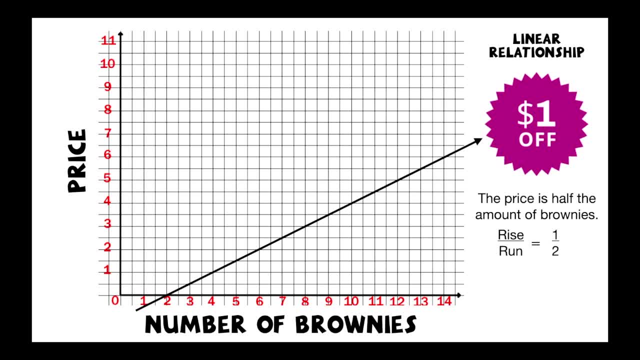 Hmm, Notice, the graph shifts. It's got to shift down to deal with that. that, that discount. but in shifting I'm still keeping the same value. I just have to make sure that I bring the price down one. So if you notice, in that ordered pair, instead of starting at zero zero, I'm now going to start at. 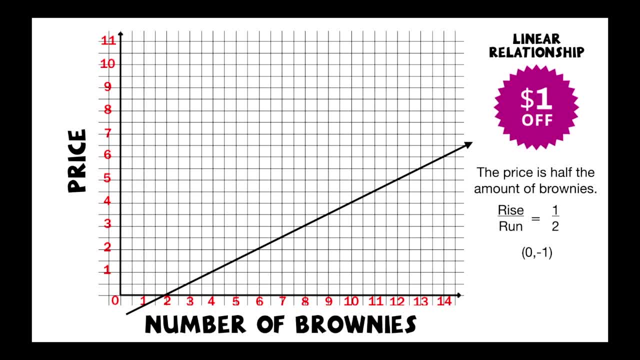 zero negative one, And that's going to denote that price of minus one, Cause I'm getting a dollar off. Okay, The price is my Y, So it's in the Y section of my ordered pair. So the point I'm really starting. 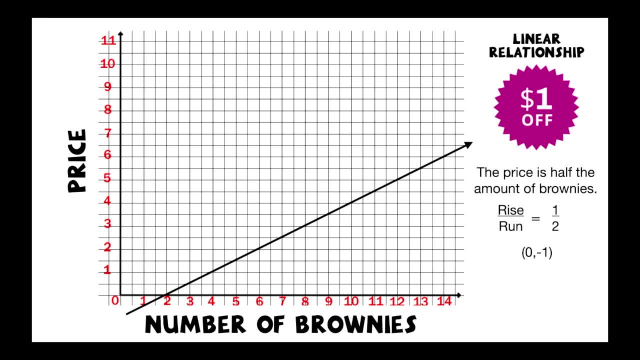 this graph at is zero, negative one, And that's going to be how I follow my pattern. My pattern is still up one over two because the value is still half, The price is still half the amount of brownies. that hasn't changed. Well, if that has changed, that now I'm getting a dollar off of the. 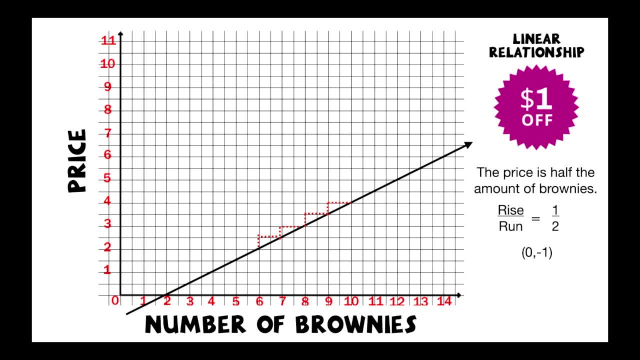 total price. Okay, Okay, How does that change my equation? Well, I know that my slope is going to stay the same, but instead of the slope just be, or the equation just being Y equals one half X, I have to account for that dollar off coupon. So it's Y equals one half X, minus one. 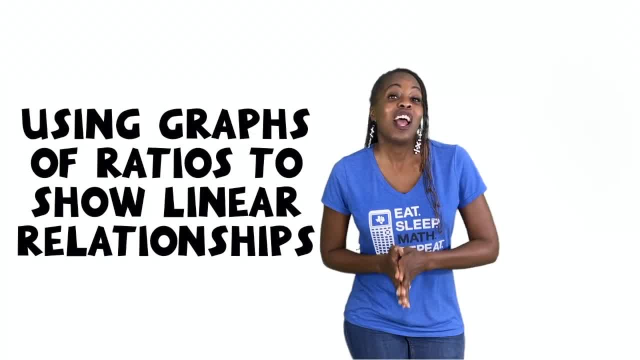 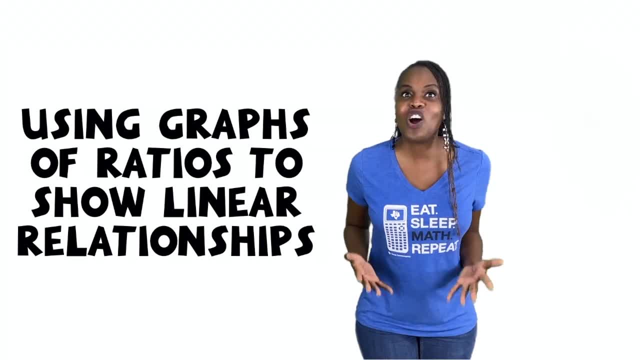 So isn't that so cool? Not only are you able to show proportional relationships through graphs, but you're also able to show proportional relationships through graphs. You can also show how proportional relationships are also linear and they have a linear relationship to them as well. Hope you liked this video. See you next time.